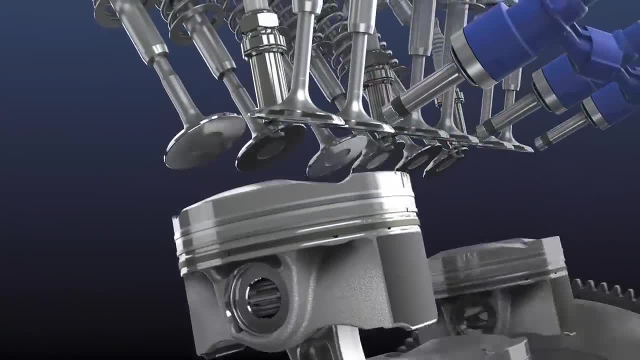 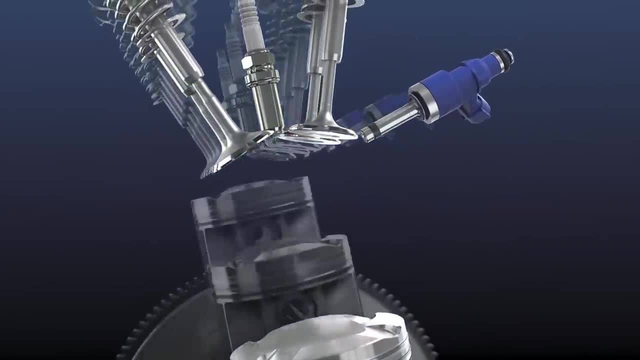 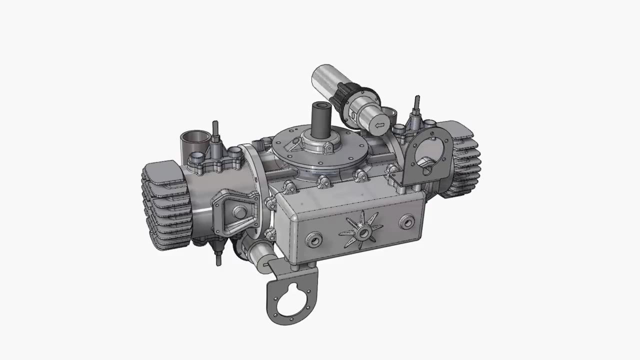 oxidized, And even if you had a gaseous fuel, you would still have problems with the components, because the detonation wave is expanding at supersonic speed. So, in reality, most piston configurations are not designed for purely controlled detonation. Having said all that, there are a couple of projects out there which are trying. 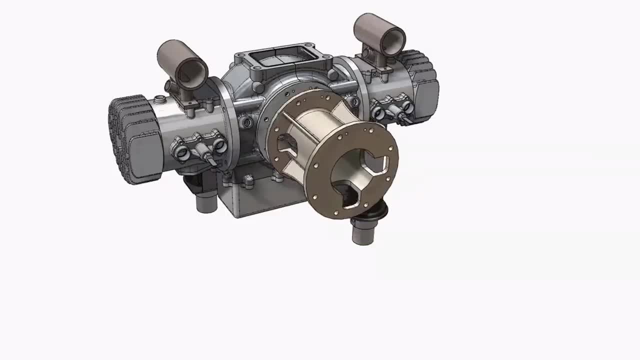 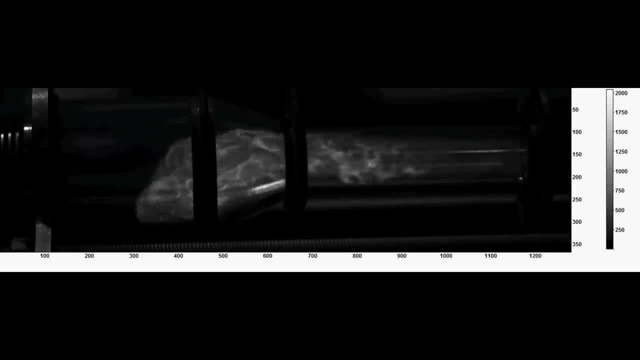 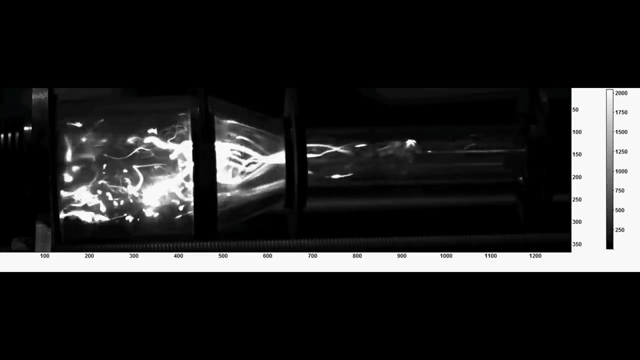 to utilize the detonation supersonic wave in an internal combustion configuration, but nothing so far has been really proven yet. A fully controlled detonation can offer substantial increases in efficiency when compared to combustion, because it is causing an explosion rather than a slow burn, And to harness this power you need a very redundant design which eliminates 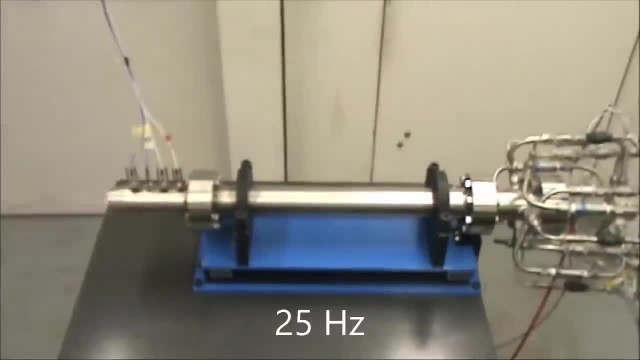 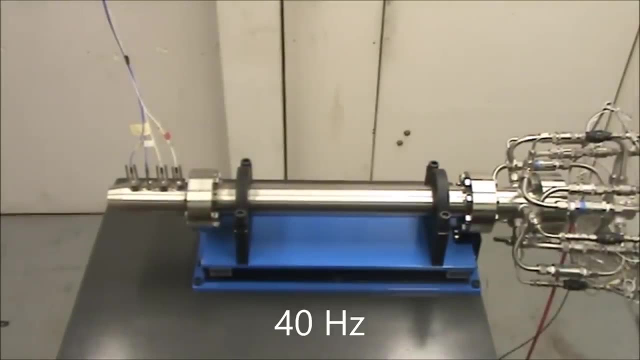 complexity. It also has to be made out of a high strength alloy which can handle these continuous explosions. So if you have a high strength alloy which can handle these continuous explosions, a pulse detonation engine can actually achieve a speed up to Mach 5.. But once again, these engines 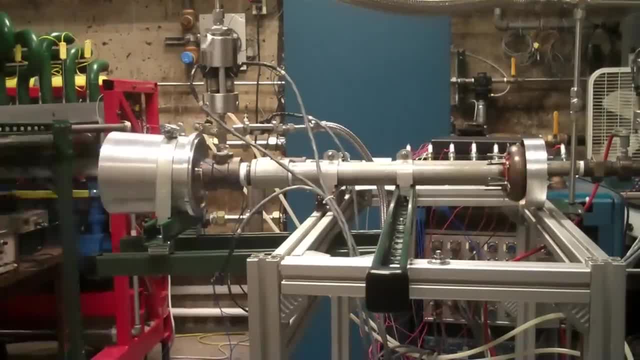 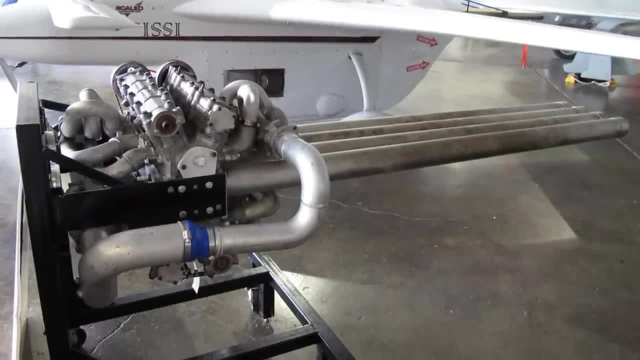 are dependent on shock waves for detonation. This causes a lot of noise and vibration, not to mention that this energy needs to be accelerated down a very long tube so that it can reach a detonation point. The next logical step would be able to control the detonation earlier. 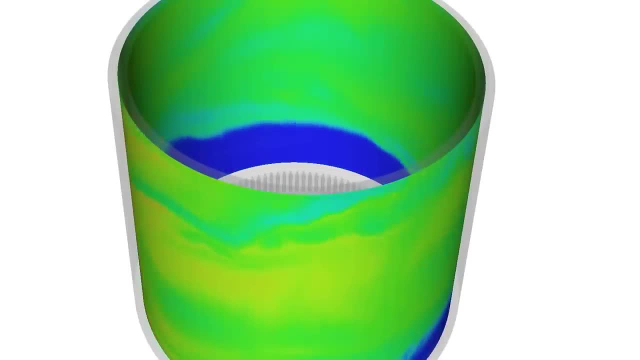 maybe even having multiple detonations happening all at once. So one way to control all this is through rotary detonation, And you can kind of think of this as a one continuous exploding tornado. Fuel and oxidizers are channeled through small holes which are then ignited by the circling. 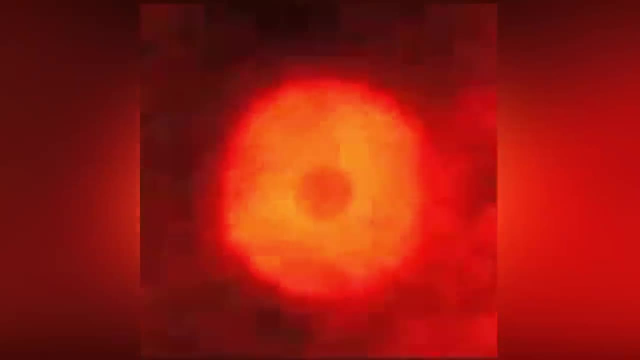 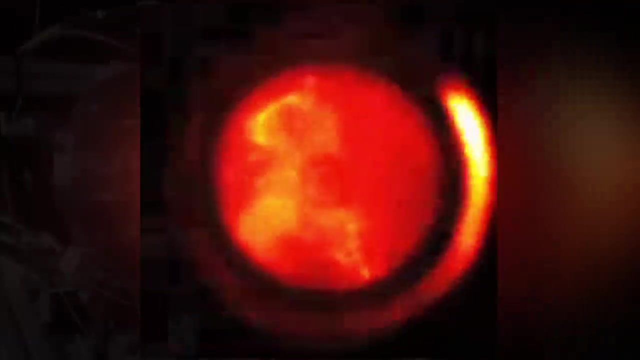 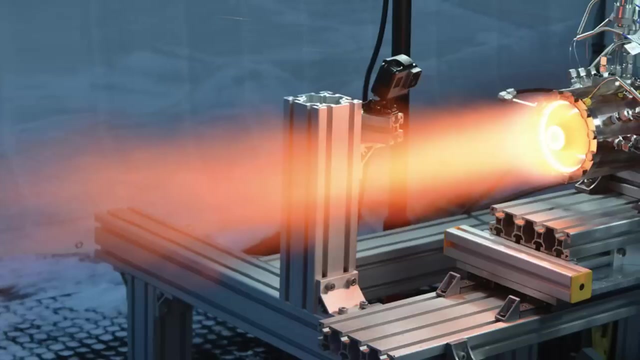 detonation wave. The result is an engine that can provide continuous thrust rather than in pulses. An RDT increases pressure during detonation, whereas a traditional jet engine sees a total pressure loss during combustion. So in theory it can be made significantly smaller than a typical jet. 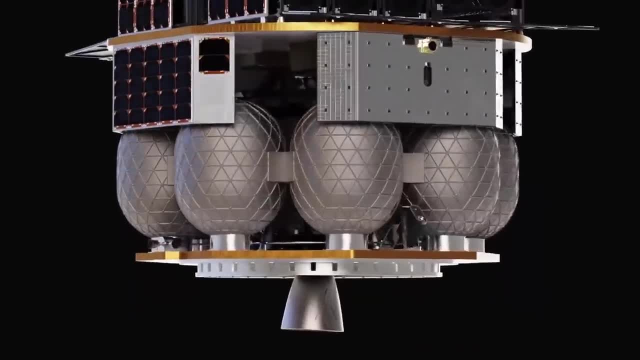 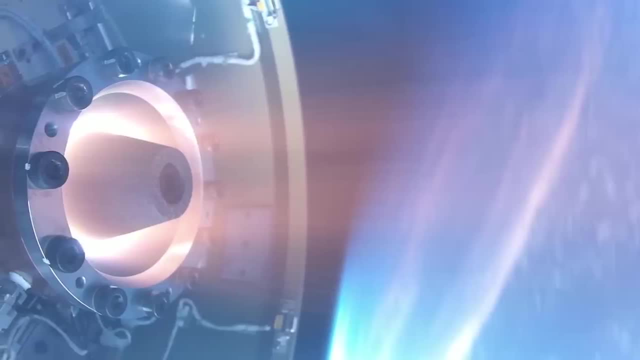 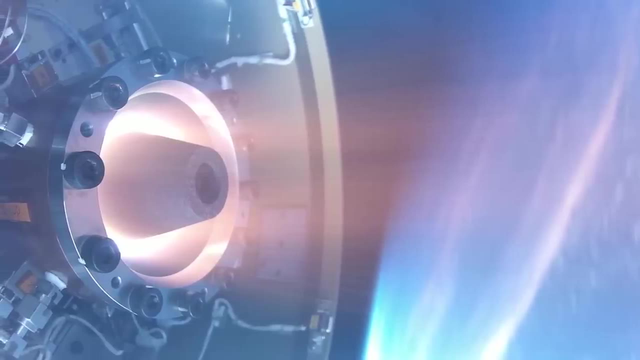 But RDE's can also replace smaller rocket engines. Unlike conventional rocket engines which require turbo pumps and very high pressure lines, an RDE simply utilizes its shock wave for pressure. Theoretically, it could reduce a rocket's weight by up to 30% with a far less complex design. 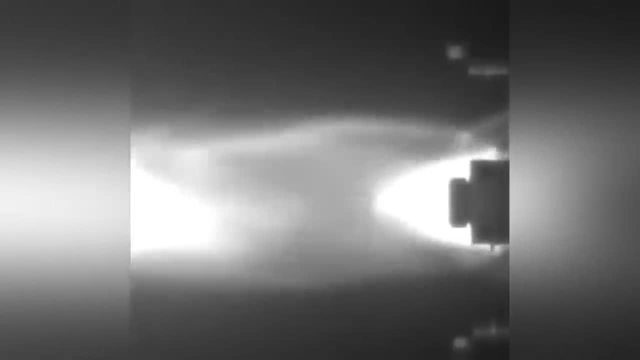 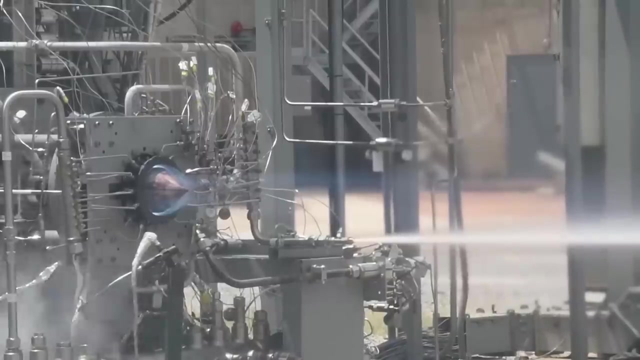 But the problem with an RDE is that it's very similar to the pulse detonation, where it's very difficult to contain these explosions in a controlled manner. But a new breakthrough is happening: It's the pulse detonation. The pulse detonation is the pulse detonation.